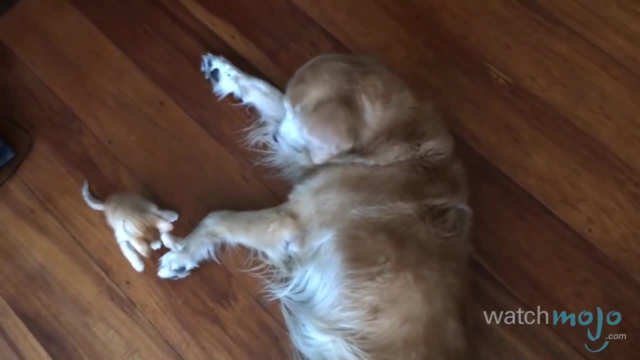 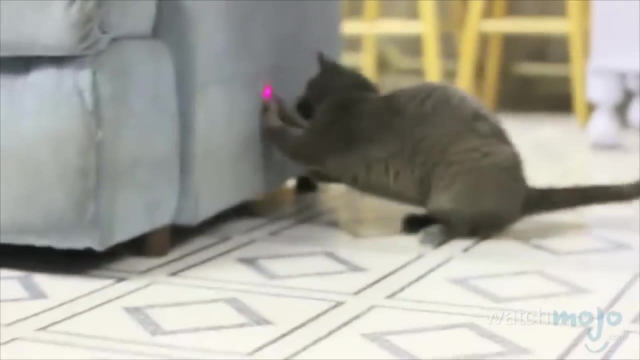 That can either be a bad thing or a good thing, because if you've got a busy lifestyle and are always on the go, a more self-sufficient animal may be a better choice for you In light of their relatively low income and low maintenance nature. 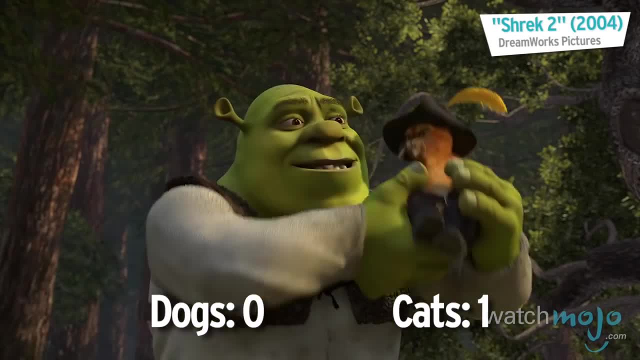 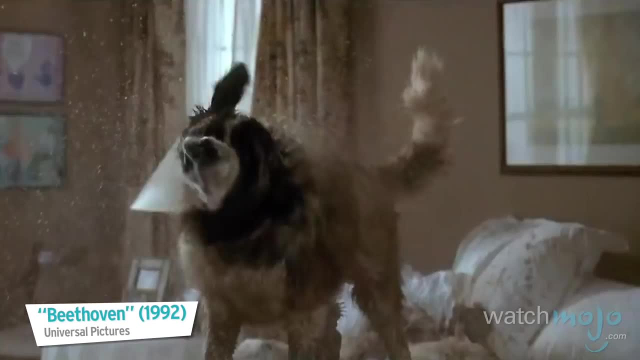 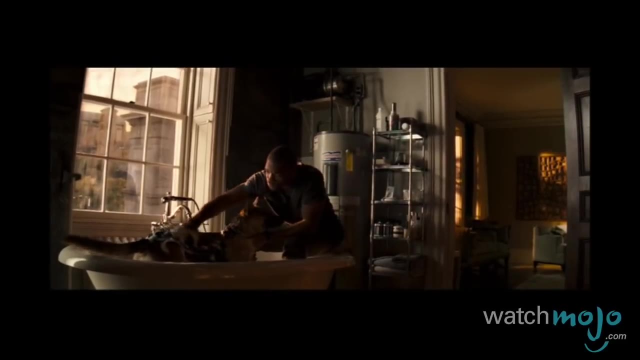 we give the cats this point. Cats, Aw, listen. he's purring. Oh, so now it's cute Round Two: Cleanliness. As with humans, pet hygiene is crucial and there are clear distinctions in how cats and dogs are kept clean. 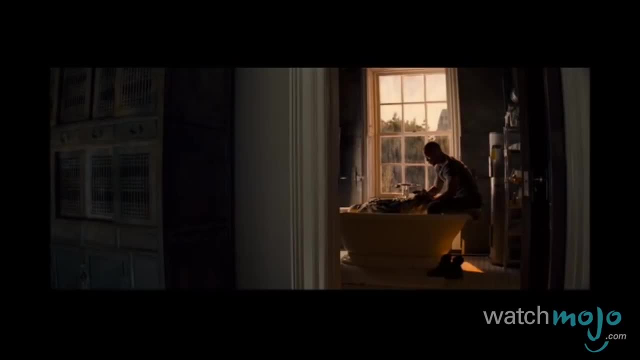 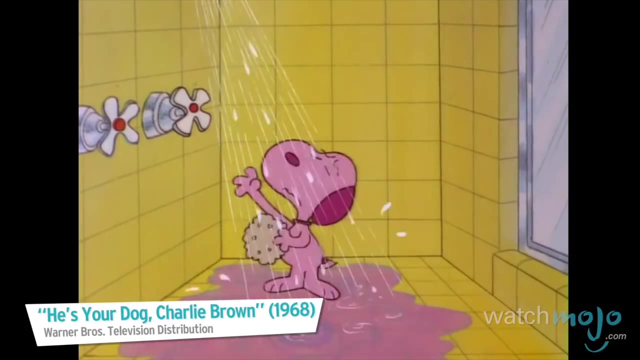 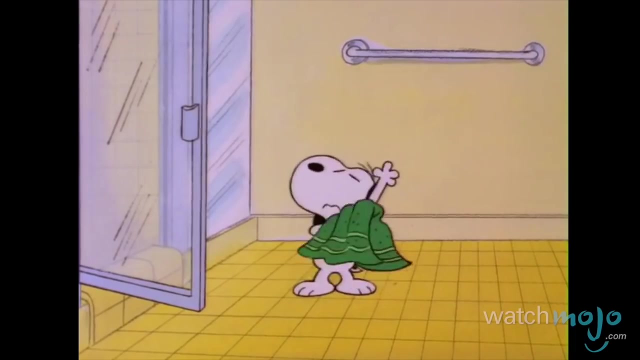 Many dogs require constant upkeep, Though the frequency varies from breed to breed, owners should ensure their dogs are bathed and groomed on a constant basis. Contrary to popular belief, not all dogs can swim or even like water, so it's not always easy getting them into the bath. 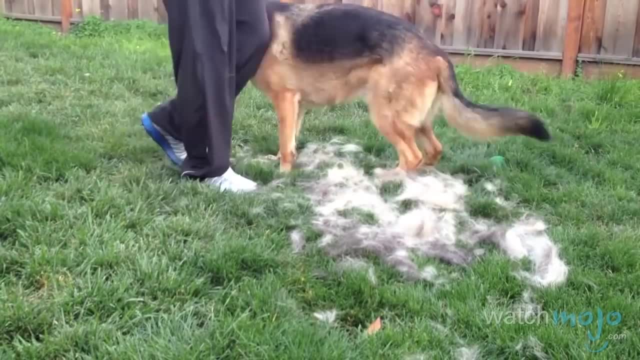 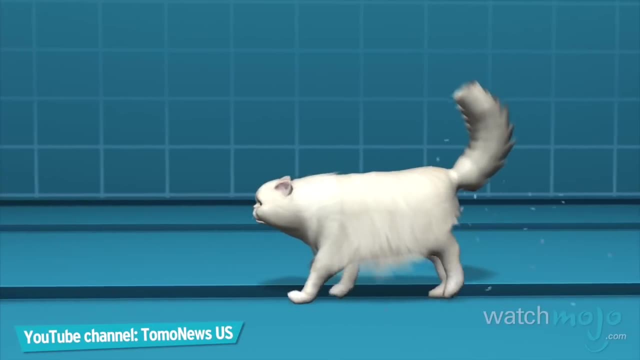 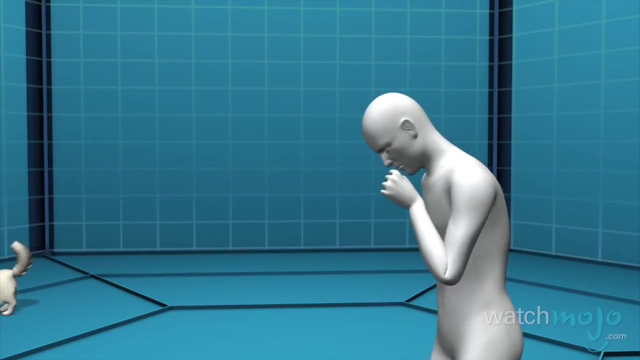 And if you've got a long-haired dog, beware of shedding and allergies, not to mention tangles, if you don't maintain your pooch, Felines of course also shed and can also trigger allergies. In fact, cat allergies are twice as common as dog allergies. And while you won't find any fully hypoallergenic cats, there are some steps you can take to lessen the symptoms. As for maintenance, cats as a rule do not require bathing, as they lick themselves and even other cats regularly. 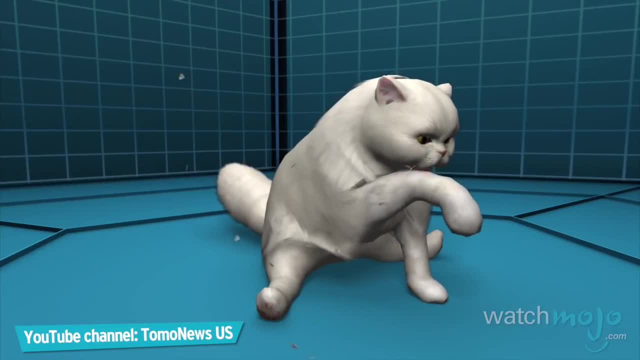 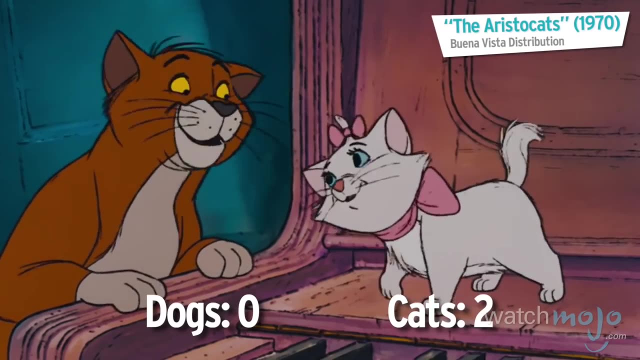 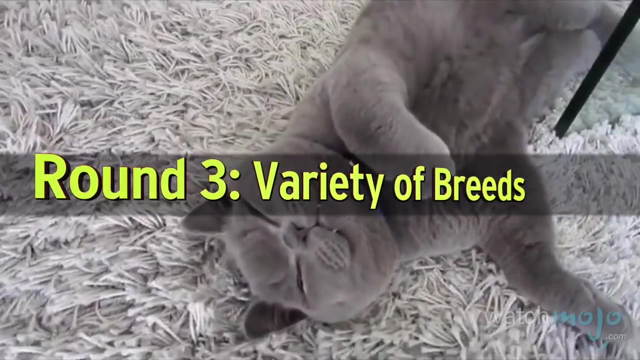 Though it is suggested that long-haired cats be brushed regularly, Based on their general ability to remain clean, cats win the round. Cats: Everybody wants to be a cat, Because a cat's the only cat who knows where it's at Round Three. 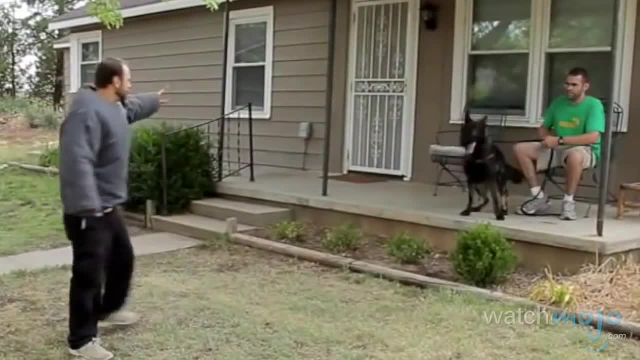 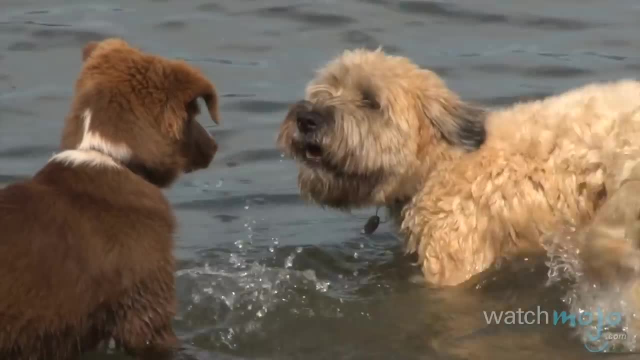 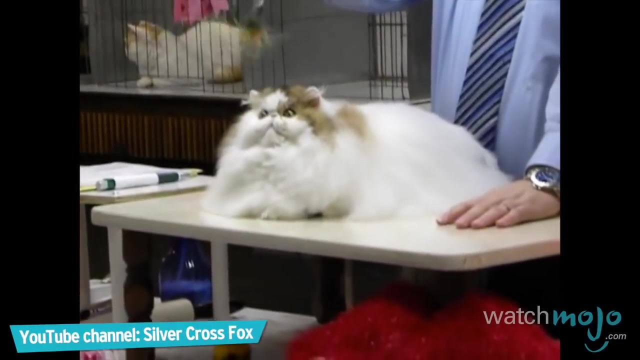 Variety of Breeds. Both dogs and cats offer a plethora of breeds for potential owners to choose from. Big or small, self-sufficient or in need of attention, there's something for everyone in both cats and dogs. Some of the most popular breeds of cats include: 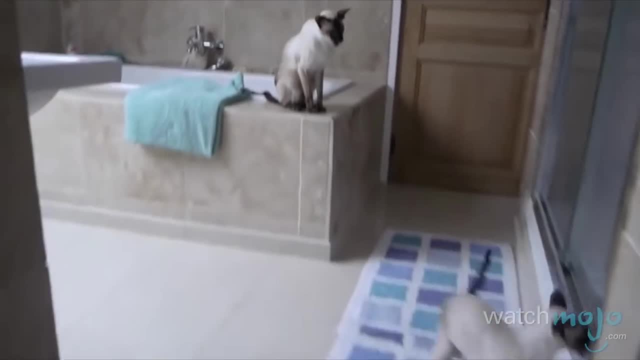 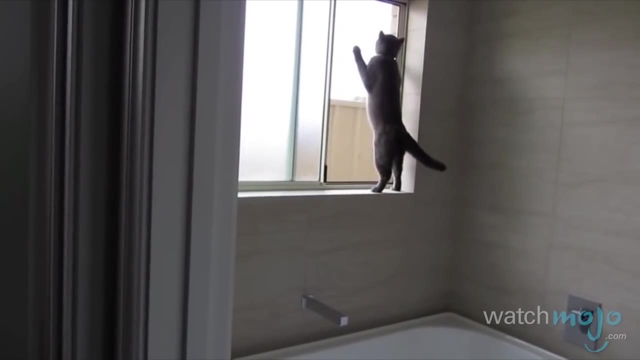 high-maintenance Persian, highly social and athletic Siamese, winter-friendly Maine Coon and the British Shorthair. But regardless of the breed, cats remain small across the board. Dogs are the most popular breed in the world. Dogs are the most popular breed in the world. 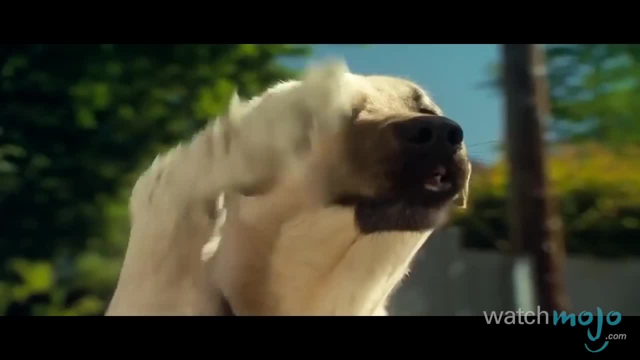 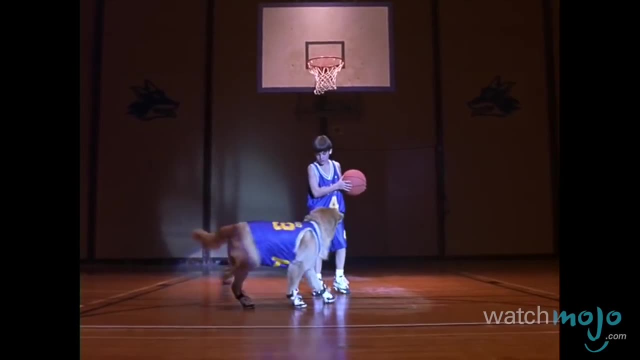 Dogs vary even more wildly, from the tall Great Danes to the tiny Pomeranians. Even among medium-sized dogs, the variation between breeds such as devoted Golden Retrievers, highly trainable German Shepherds and attention-loving Bulldogs is quite astounding. 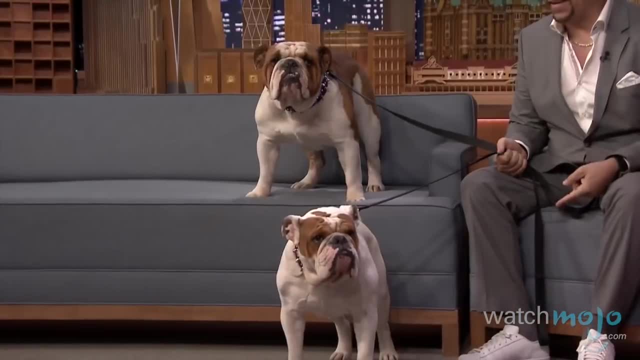 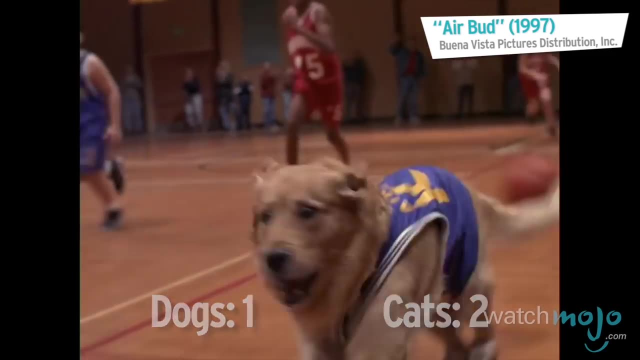 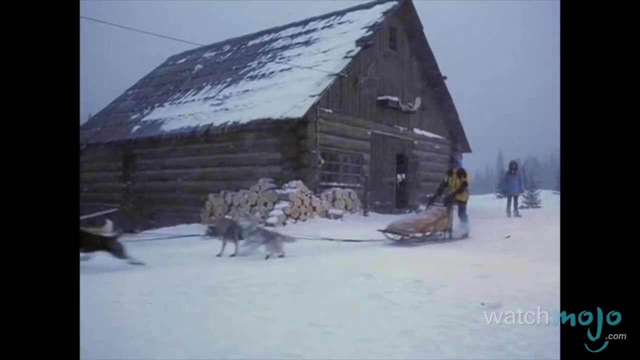 How they're just looking right in camera. They're camera-rated. They like what's up, Given the great diversity of breeds available- dogs- take the point Dogs- Will somebody cover the dogs Round four Functionality In addition to house training and tricks. 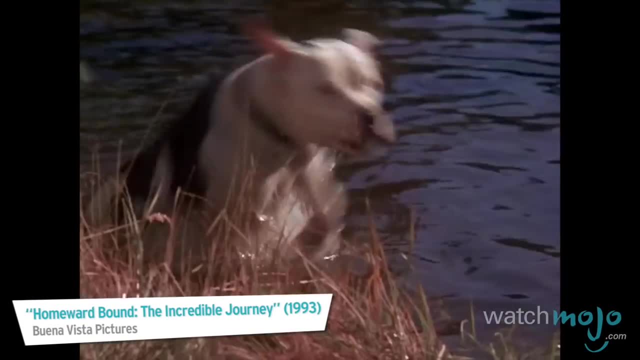 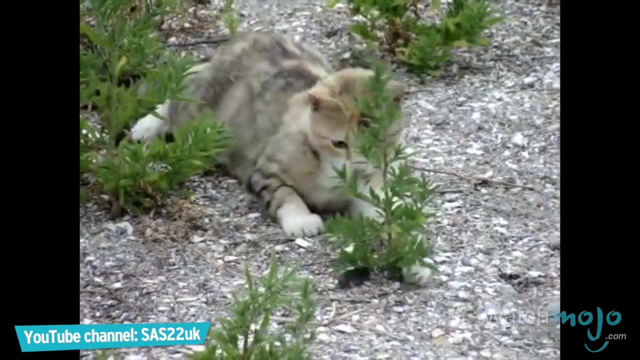 the topic of function is not uncommon when it comes to cats and dogs. Each is uniquely suited to certain tasks and purposes. Cats are well-known for their hunting and killing of rodents, generally being effective at driving out mice, rats and other animals of the sort. 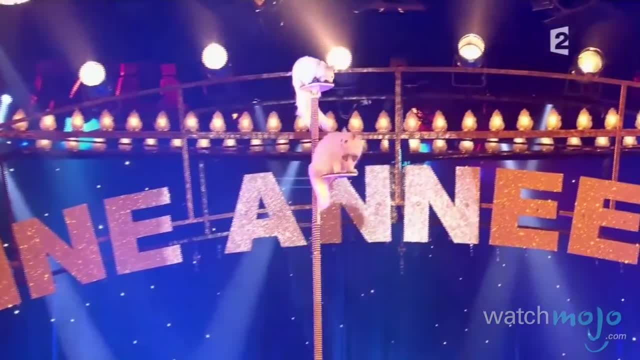 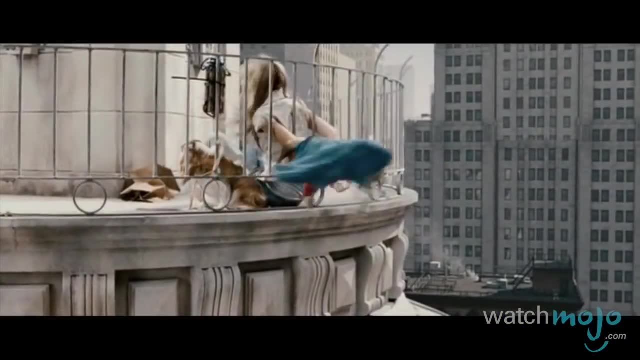 However, their skill set doesn't extend far beyond that. In short, as mentioned, cats are usually considered more independent. Help me, Please help Somebody. help me, Help. Dogs, meanwhile, are known for their loyalty, trainability and devotedness to humans. 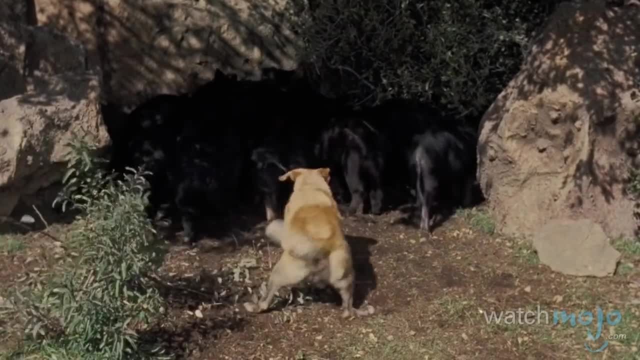 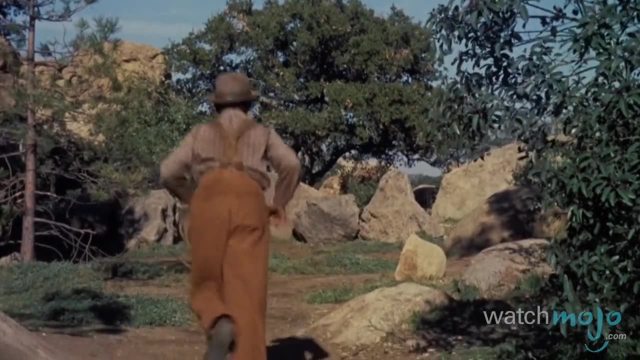 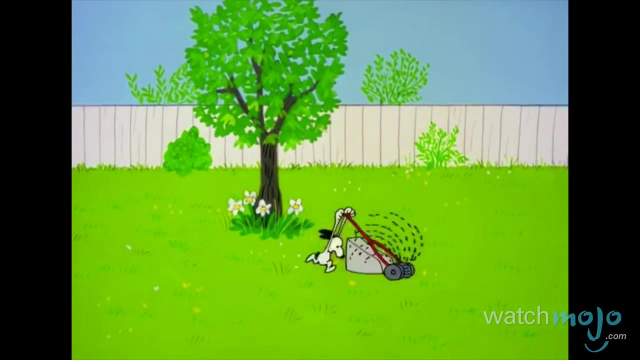 which is why they're considered man's best friend and have been trained to help humans in many ways. Pull him boy. They're routinely sought for many jobs, like sniffing out drugs for the police, acting as service dogs, assisting in hunting. 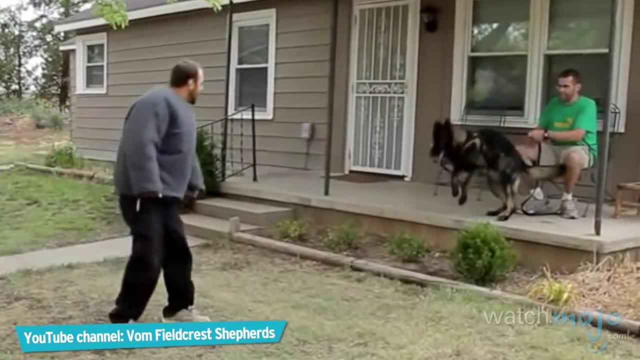 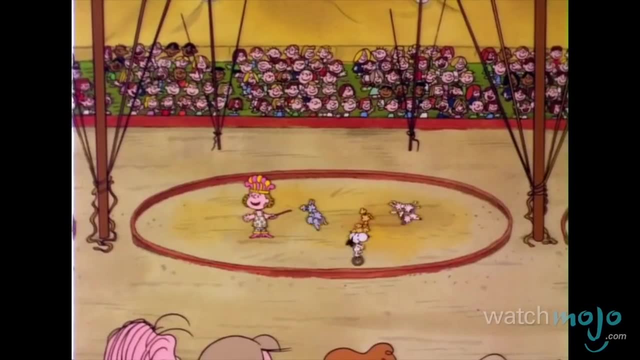 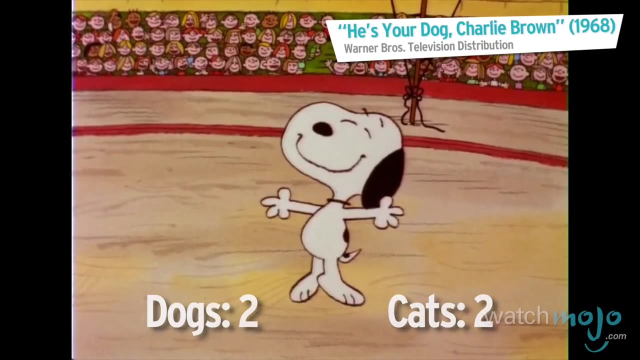 or even simply protecting their owner in the home. Yeah, what are you gonna do? Let me in your house. Come on, let me in For the multitude of roles that they can adopt. dogs win the round. Dogs Round five. 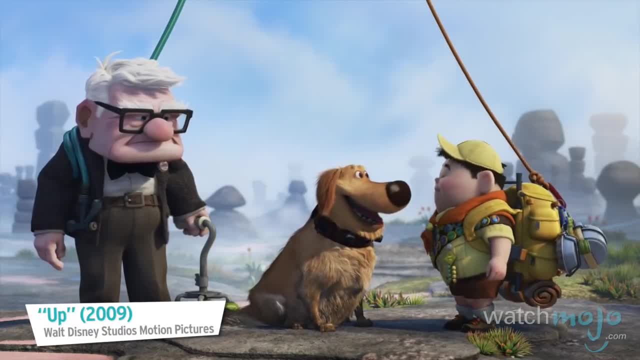 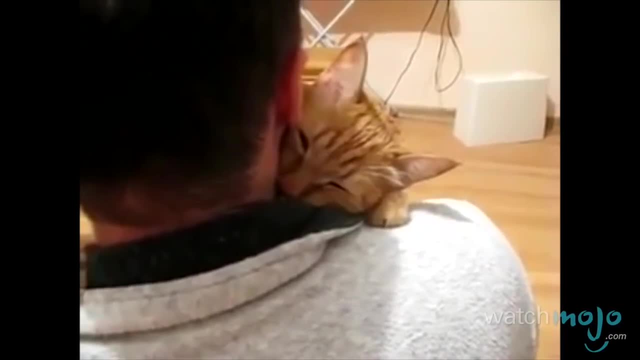 Interactivity: Shake Uh-huh, Speak Hi there. When it comes to pets, perhaps the greatest measure of their value is how they interact with their owners, both in terms of activities and where interactions occur. Cats are largely indoor-oriented. 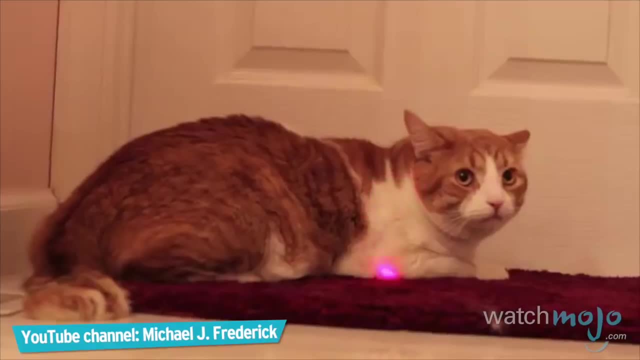 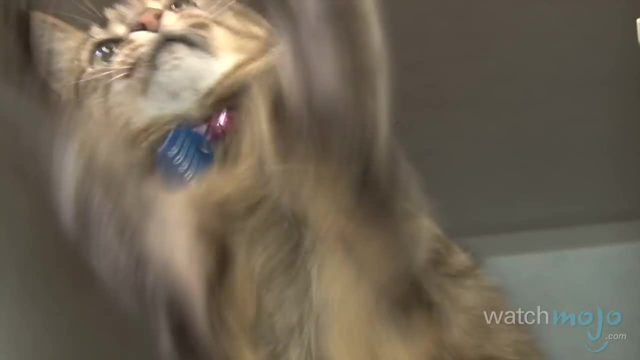 typically enjoying things on their own terms When an owner can get their attention. cats are often entranced by simple items such as laser pointers, string and yarn. They have a particular fixation on basic games that let them stalk and pounce on objects. 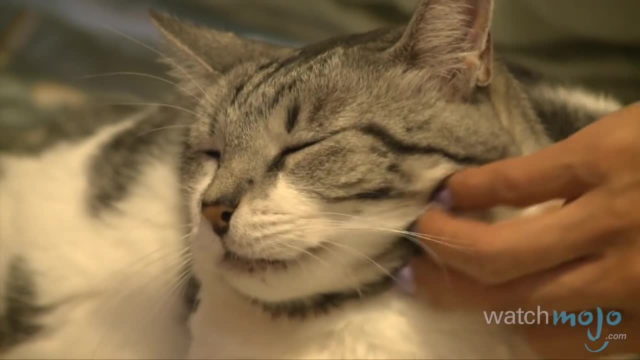 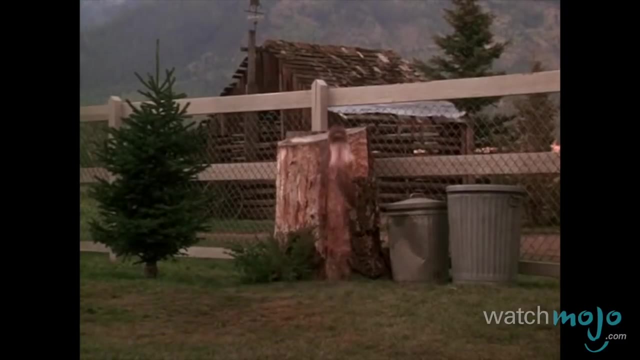 Cats do show affection. cats do show affection for their human masters and can be social creatures, But, as mentioned, they usually prefer to stay indoors, Meaning. if you like to explore the great outdoors, kitties may not be your best companion.